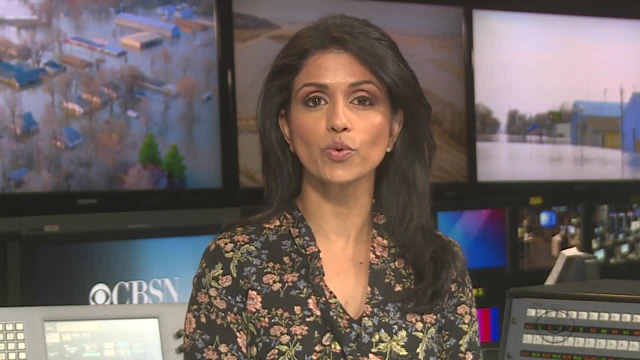 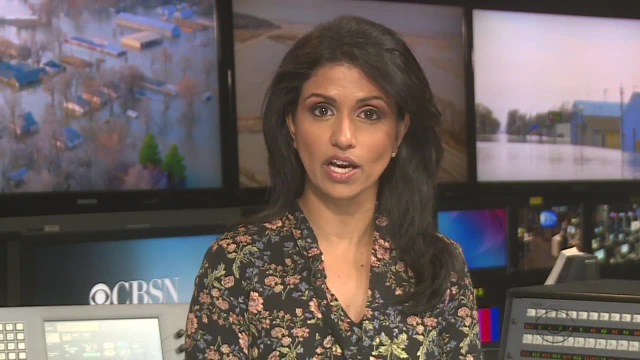 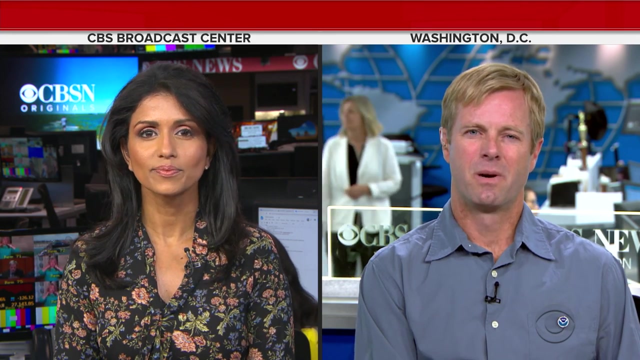 live in counties directly on the shoreline. I spoke with Dr William Sweet, an oceanographer with NOAA, about high tide flooding and how it could be a big problem for those living on the coast. What exactly is high tide flooding, or what they call sunny day flooding? Sure, well, high tide. 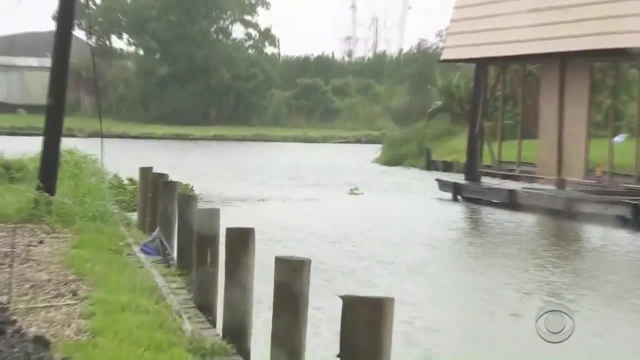 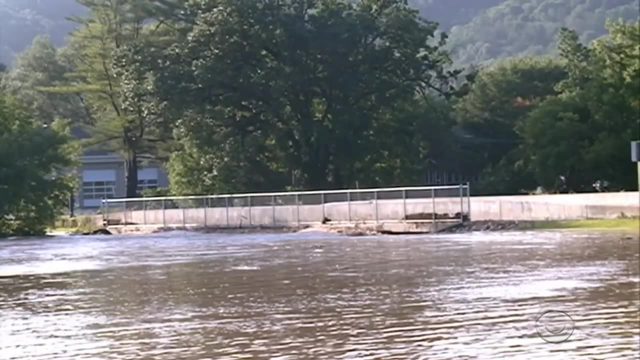 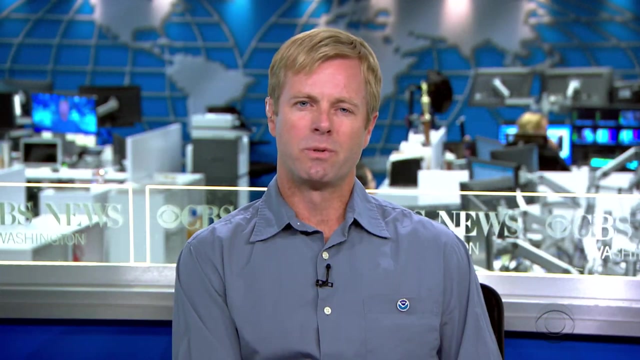 flooding is oftentimes referred to as nuisance or sunny day flooding. It's increasingly common due to years of increases in relative sea level rise. It's the kind of flooding that used to not occur decades ago, but because of sea level rise, now, full moon tides are sufficient to flow into stormwater drains and flood into streets. It's 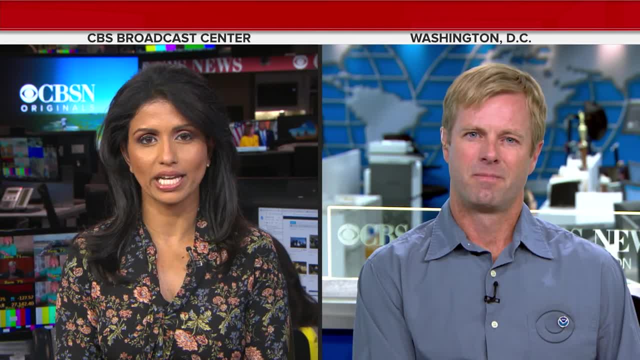 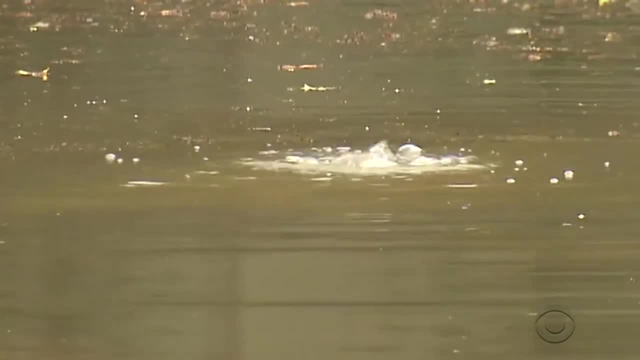 sea level rise, It's high tide flooding. So what are some of the major issues that high tide flooding can cause in coastal communities? Well, high tide flooding is mostly disruptive. It's clogging stormwater drains, It's spilling into streets, It's making people go different routes to school. 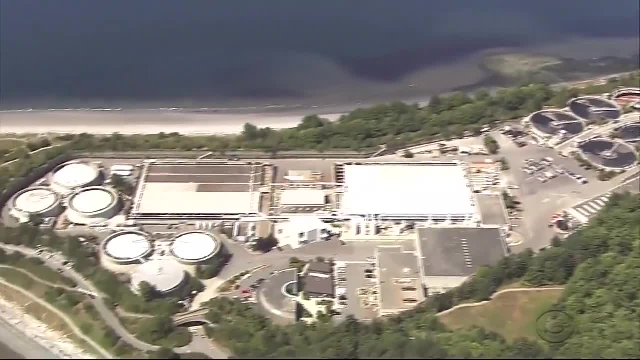 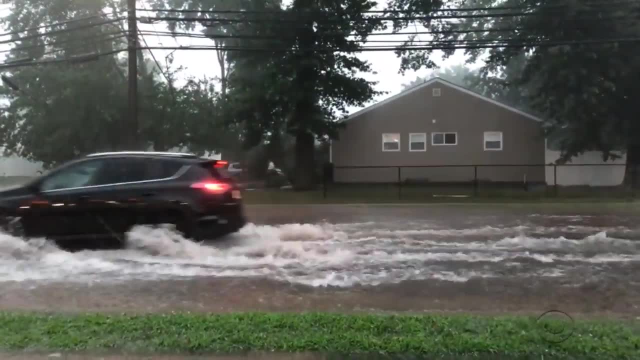 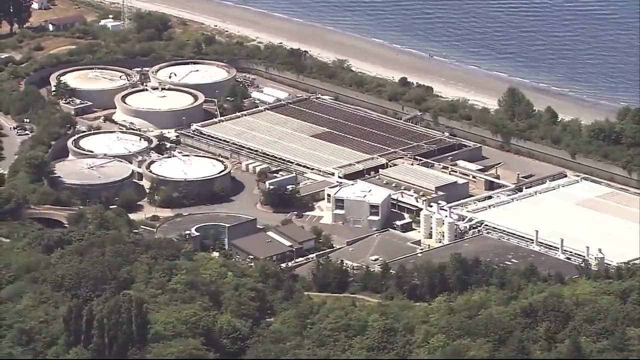 to go into different routes to church. But there's other impacts as well. There's some, as I said, problems are degraded, and that's particularly a problem if it rains too. Then there's just really no way to get water off the streets. It threatens freshwater supplies, wastewater systems, septic. 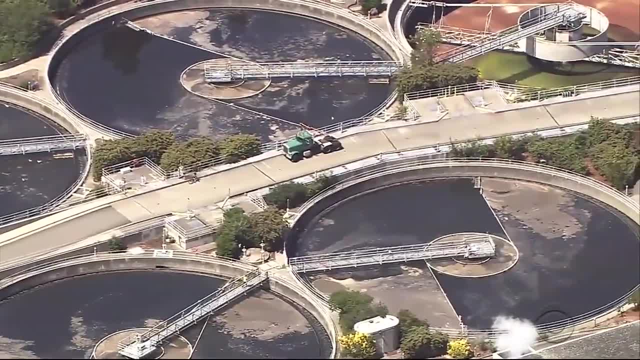 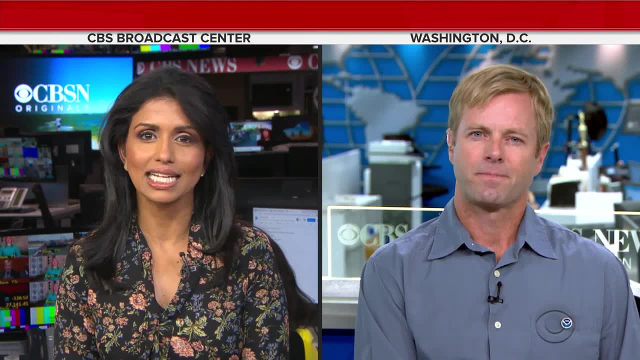 tanks. So there's really a host of concerns and problems that are surfacing right now in high tide flooding, and that's why we're monitoring and tracking the situation at NOAA. Your report projects that high tide flooding will roughly double across the US coastlines in 2019, and 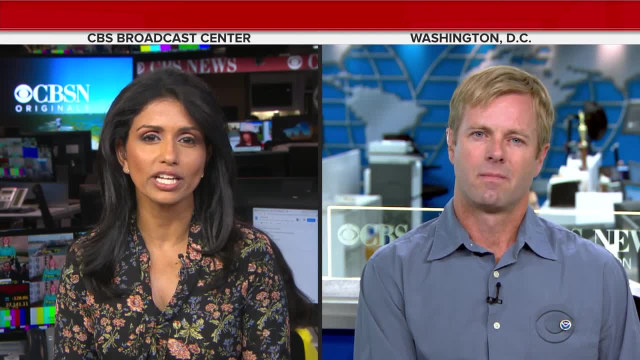 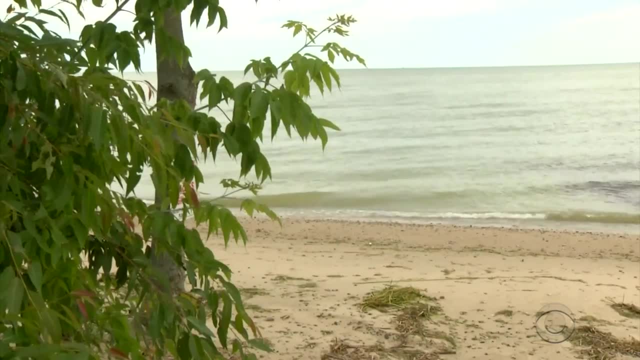 continue to increase over the next few decades. Can you give us sort of an explanation as to why that is? Well, the main reason is sea level rise. Again, due to decades worth of sea level rise, the gap is really closing between the tides and our infrastructure It used. 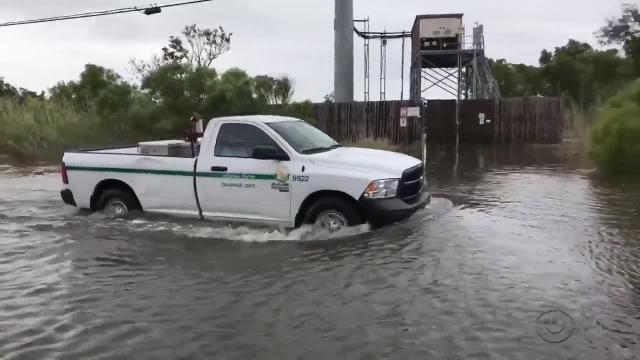 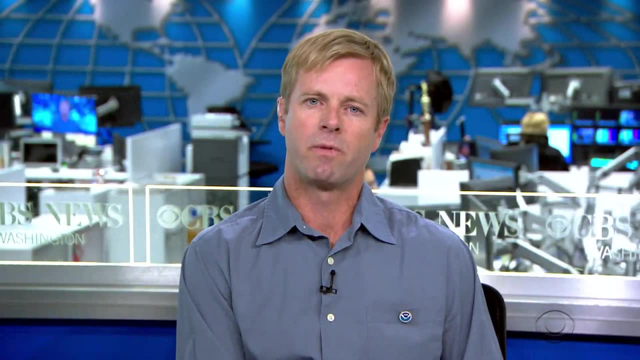 to take a localized storm to flood streets. Now it's these full moon. tides are really starting to be a problem, backflowing into stormwater systems and flowing into the streets, And so what we've documented in this report is we're trying to keep a perspective of you know how things have changed. 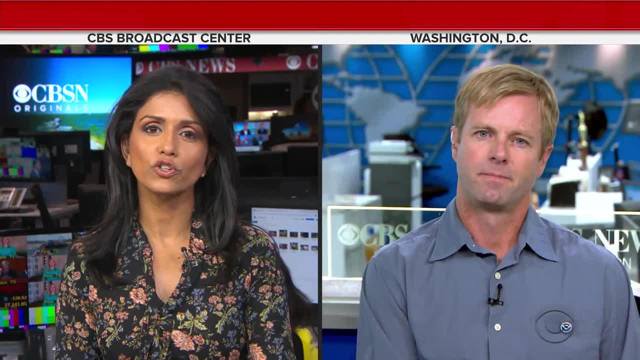 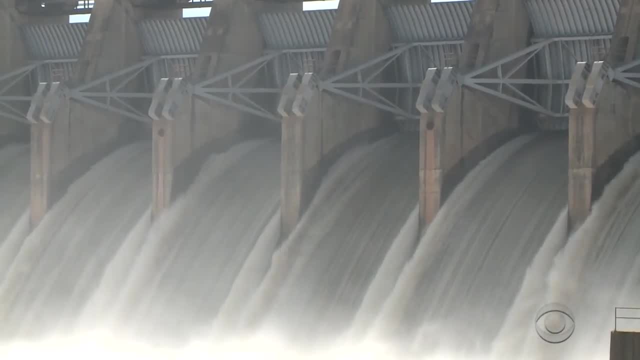 and how are they likely to change in the future, And do infrastructure systems need to be upgraded in response to the changing environment? Well, yes, the short answer is they do. The stormwater systems in particular, through the combination of sea level rise and high tide flooding, and with 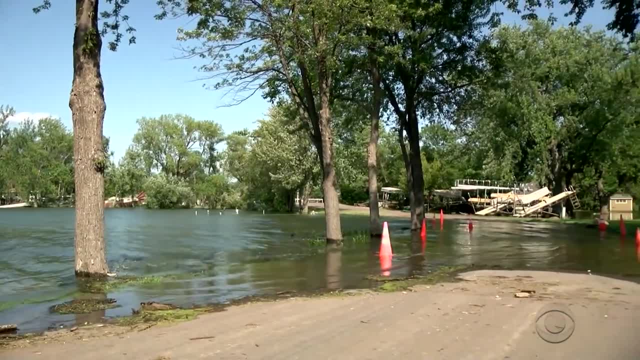 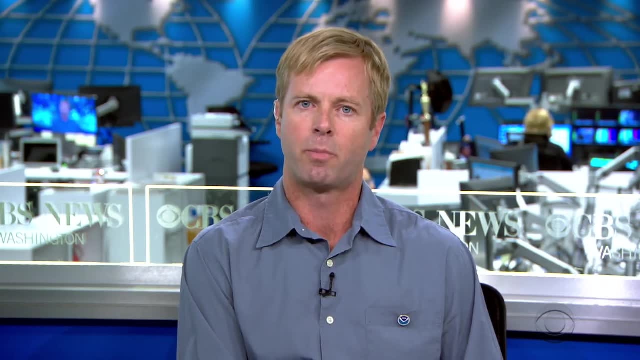 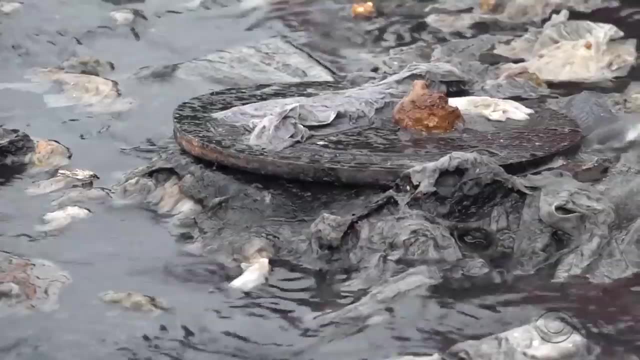 heavier rains. many communities are just finding that they're actually flooding, quite often sufficiently enough that they're actually spending money to actually upgrade and defend against these kind of problems, Installing pump systems that actually actively remove the water where these downhill gradient of the old stormwater systems of 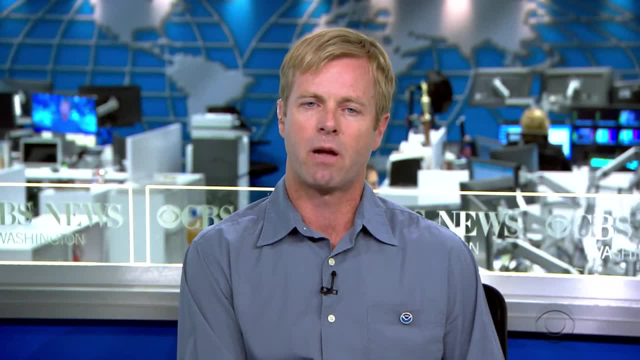 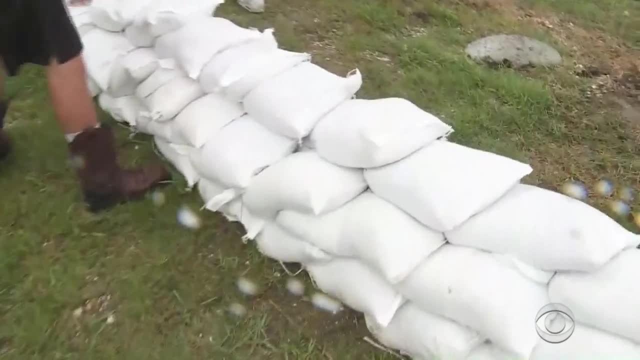 yesterday just aren't able to clear the water. So that's sort of the ground zero is water where it used to not be and now it is, As well as then. also the fortifying against the big storms, the hurricanes, as well as the lesser storms, both prove fruitful in really defending against this. 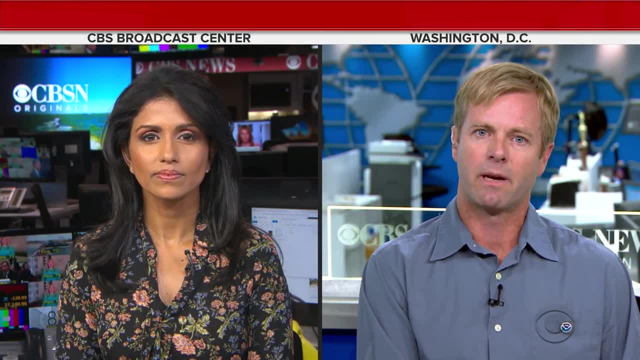 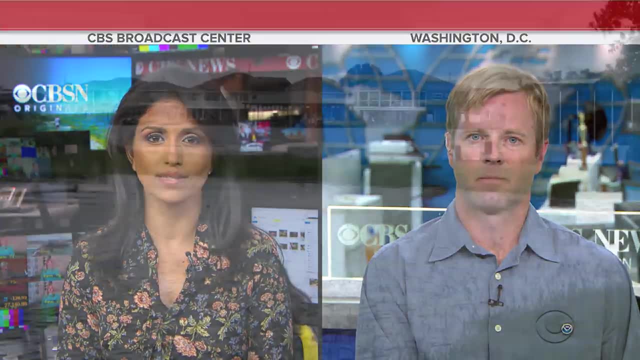 getting critical infrastructure off the ground and recognizing, you know, the vulnerabilities today so you can defend against those for tomorrow. How concerned should we be? Can anything be done to reverse these trends? Well, it should be concerning. You know, the national rate of high tide flooding has doubled. 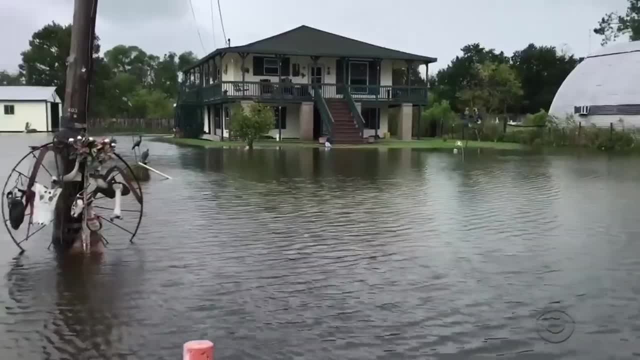 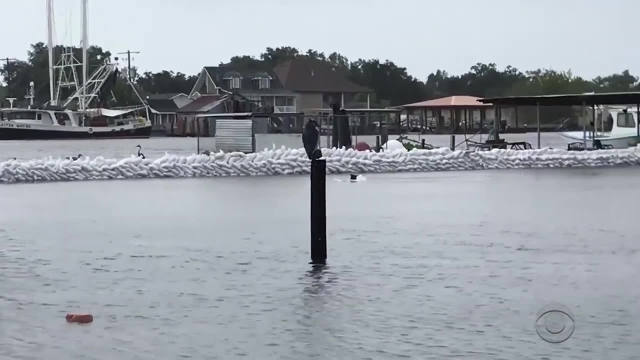 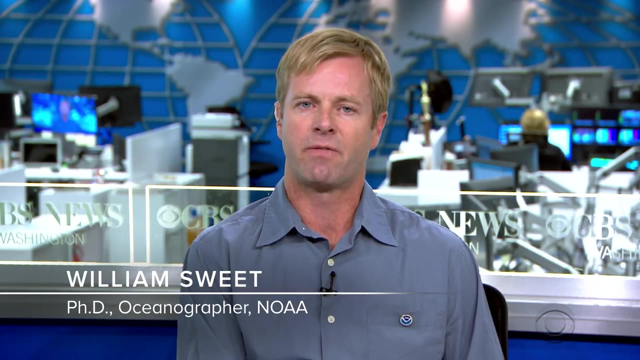 in the last 20 years or since 2000.. When we look to the future, by 2050, the rate of high tide flooding is likely to be five to 15 times greater than it is today. So for a local perspective, somewhere like Norfolk, Virginia, typically would experience five days of high tide flooding in. around 2000,, mostly from storms. Last year had about 10 days of high tide flooding in a combination of storms and sunny day conditions. In 2050, those rates are expected to really amplify upwards of 60 to 170 days of high. 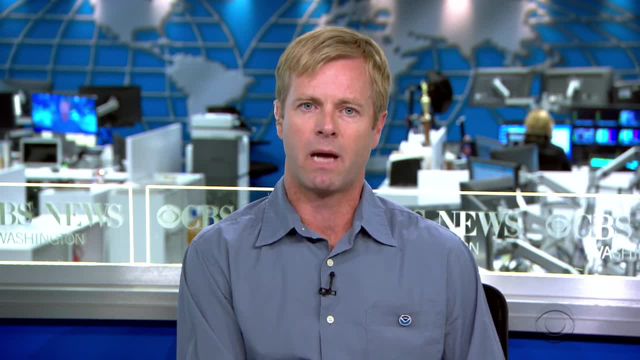 tide flooding. So it really is a problem, not just in Norfolk but many east and Gulf Coast communities, And it's something that there's time to plan and change, And what we're doing at NOAA is providing the science and services so these communities can plan and pair. 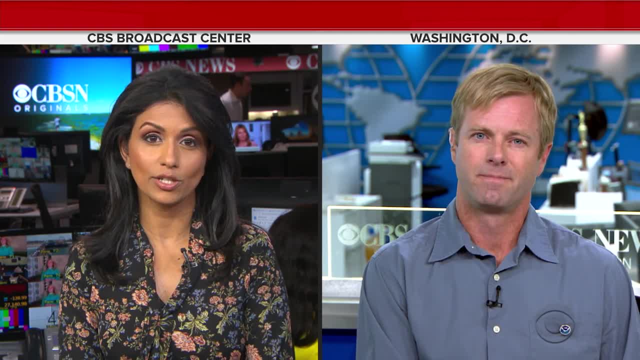 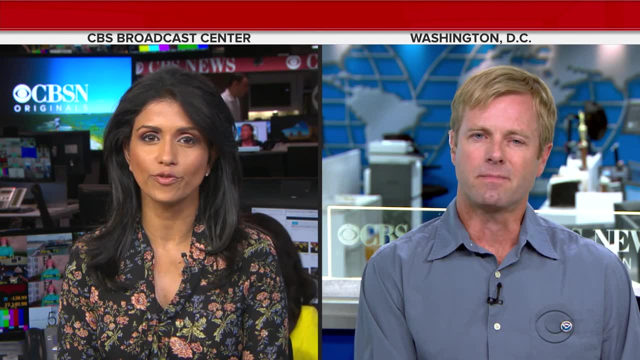 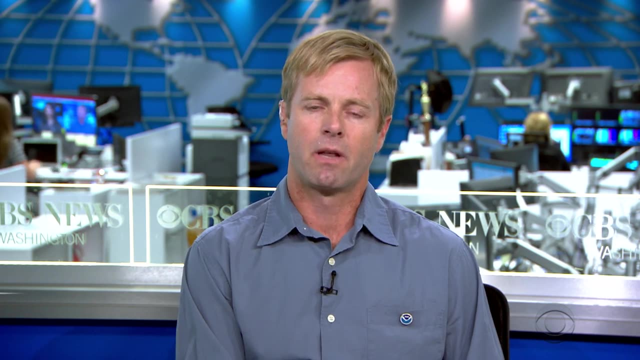 prepare accordingly for future changes. And finally, William, when considering the issue of climate change for future generations, what message should we be conveying about the need for awareness, the need for preparation for a changing environment? Well, I think it's important to recognize that change is at hand now. Sea level rise impacts are